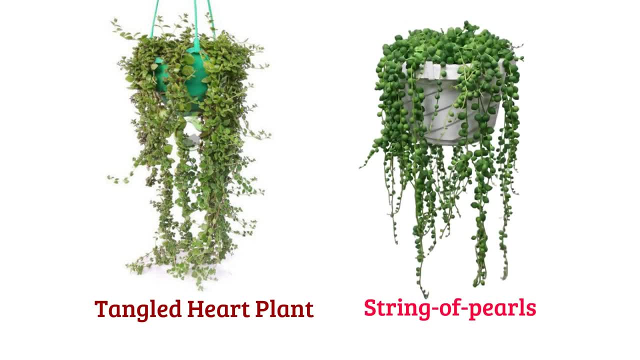 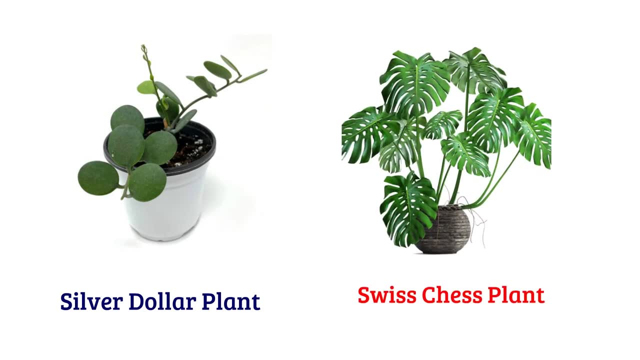 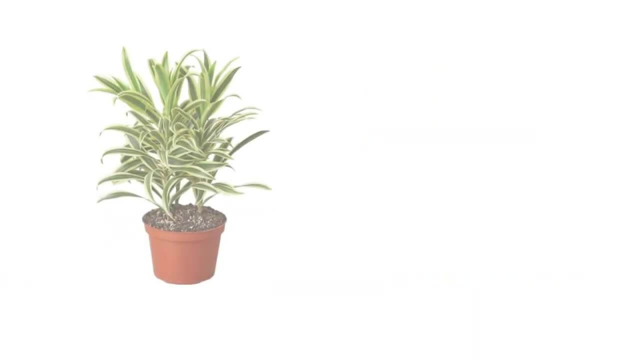 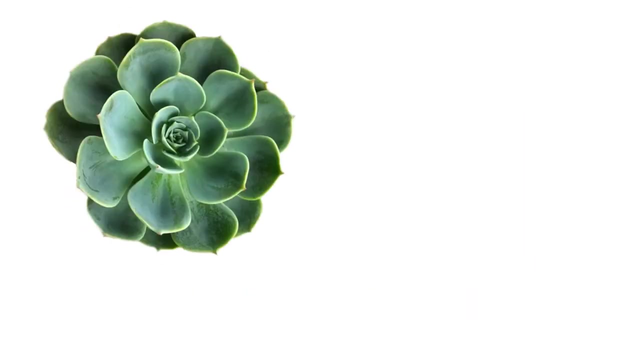 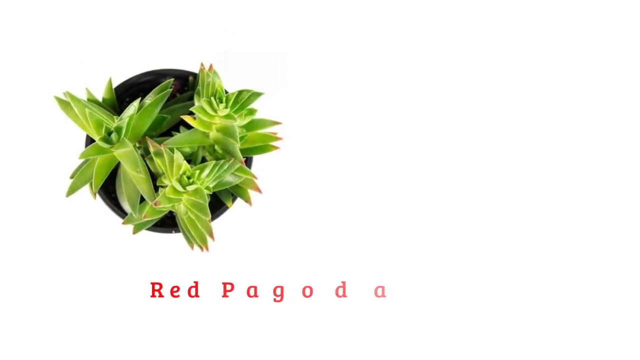 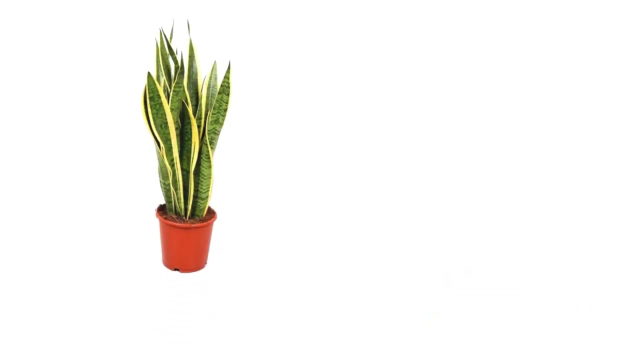 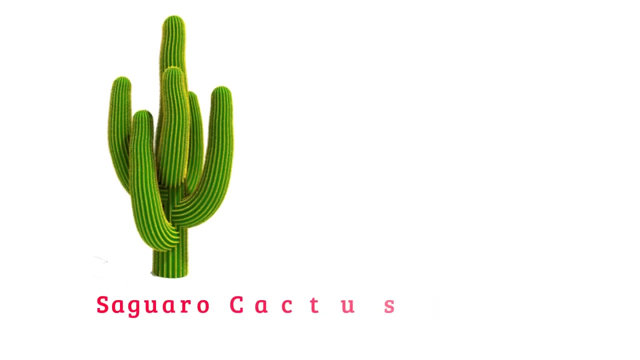 Tangled Heart Plant. String of Pearls, Silver Dollar Plant, Swiss Chess Plant, Spider Plant, Dracaena, Song of India. Rubber Plant, Achiveria, Queen Victoria, Agave, Red Pagoda Sky Plant or Air Plant, Snake Plant, Rattlesnake Plant, Saguaro Cactus. 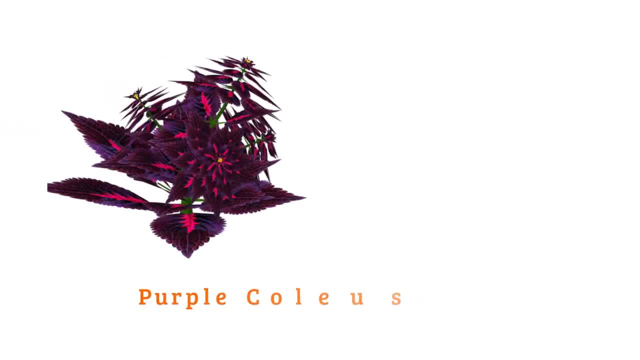 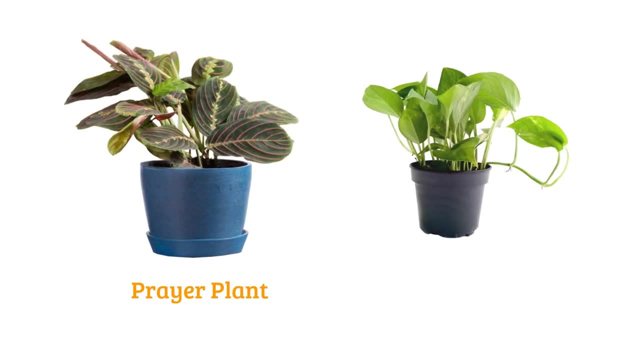 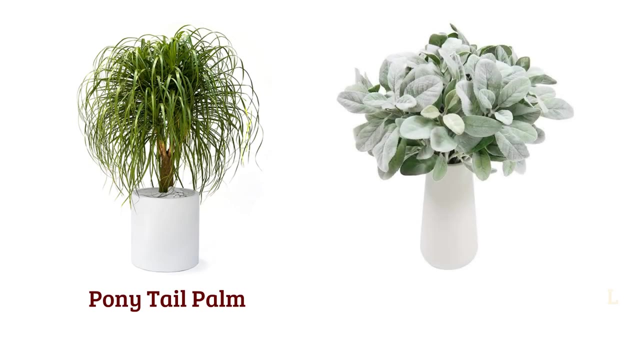 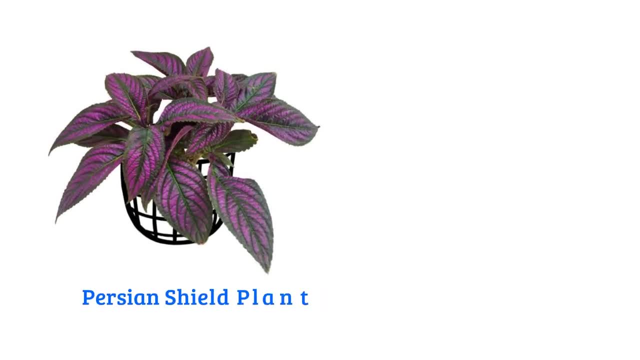 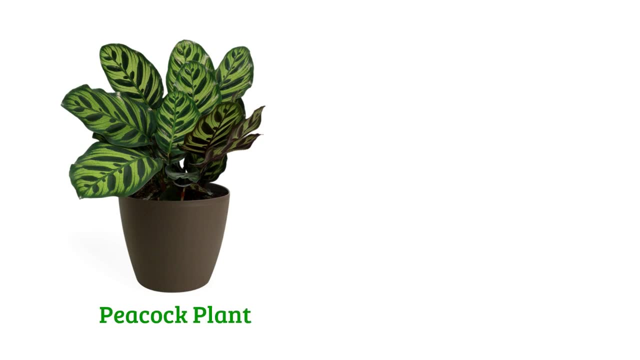 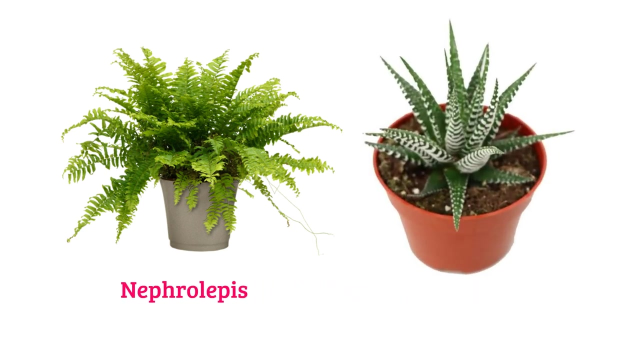 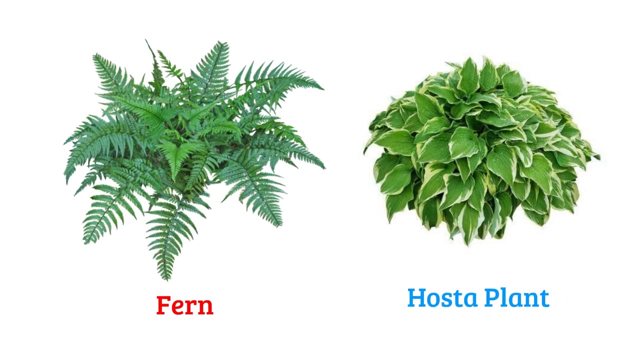 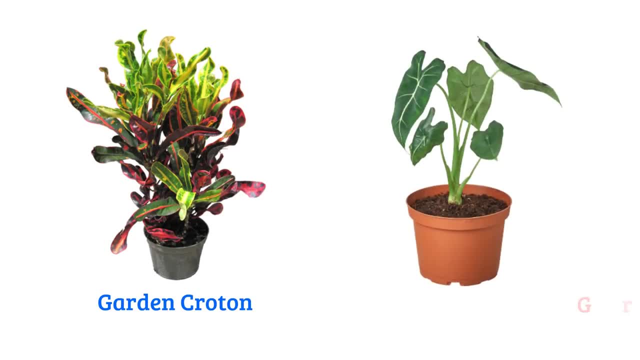 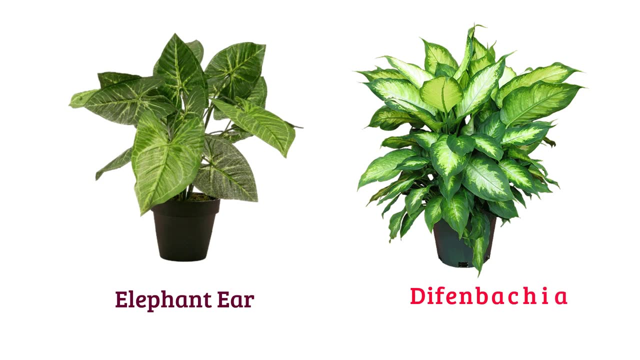 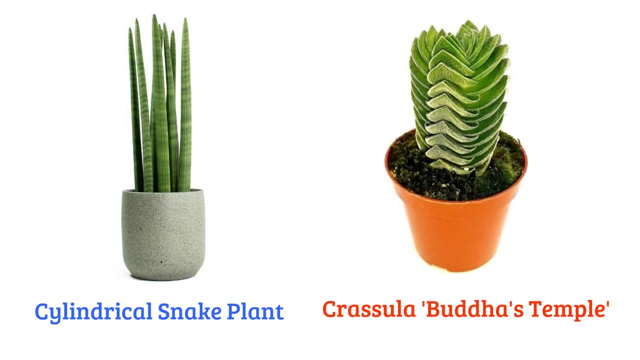 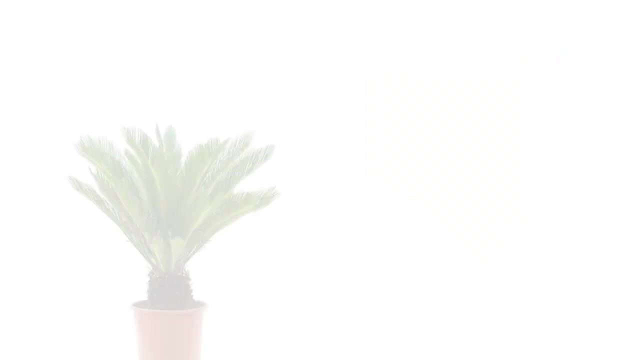 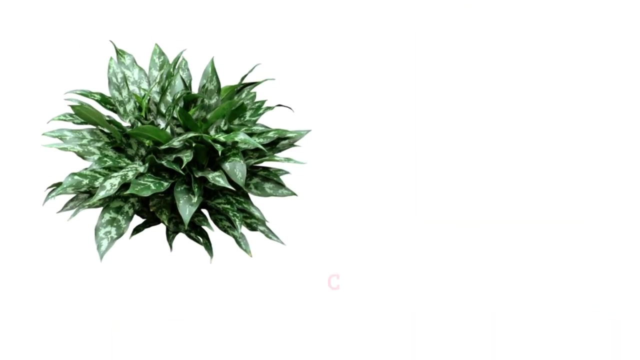 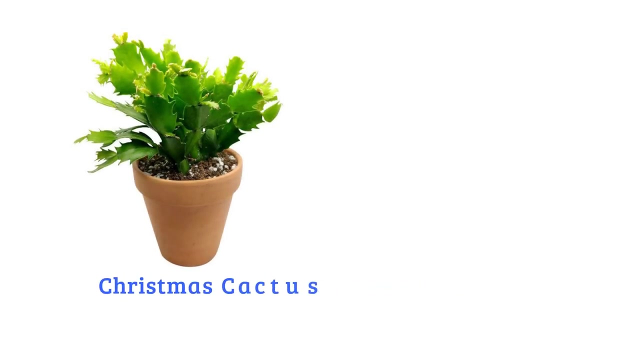 Garden. Croton Green, Velvet Alocasia, Elephant. Ear Diphonbechia Cylindrical Snake Plant. Crassula Buddhas Temple Croton. Coleus Sycas Plant. Arika Palm. Chinese Evergreen Agave- Christmas Cactus. 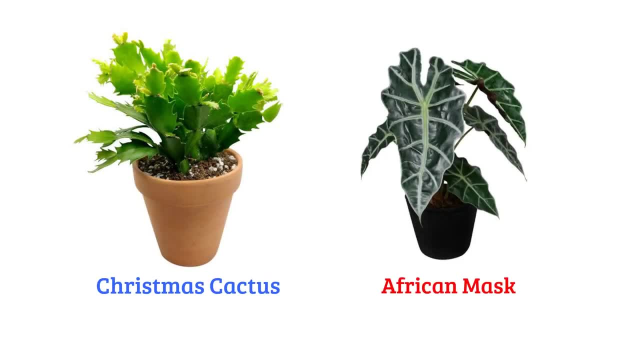 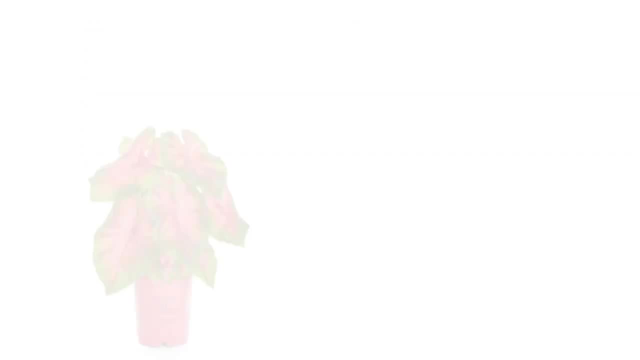 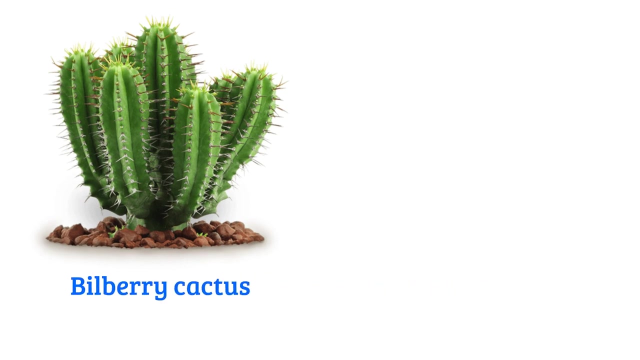 African Musk Cast Iron Iron Plant, Broadleaf Lady, Palm Caladium Plant, Aglaonema Bucksoot Plant, Bansai Burostel Plant, Arborvitae Bilberry Cactus, Bagonia Plant. 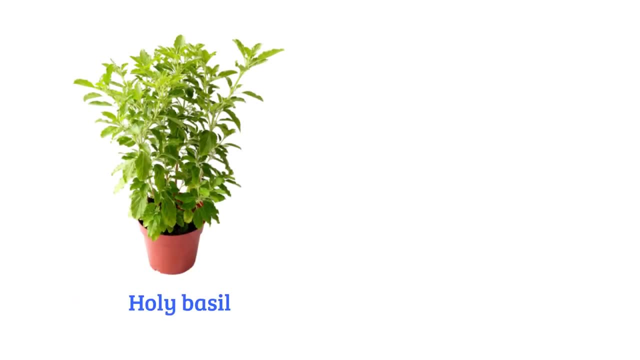 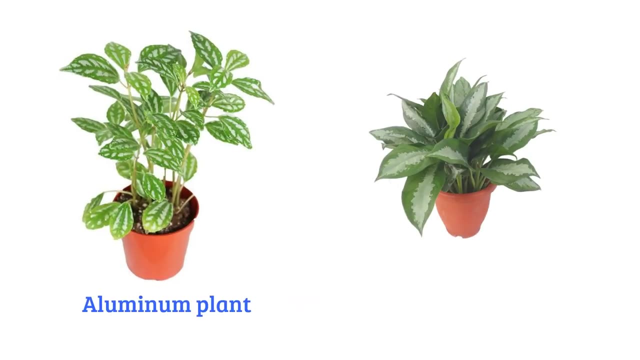 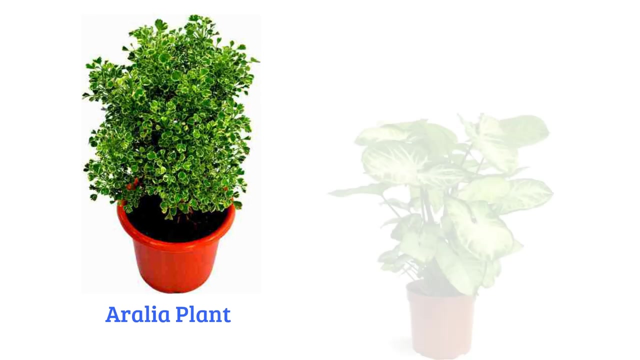 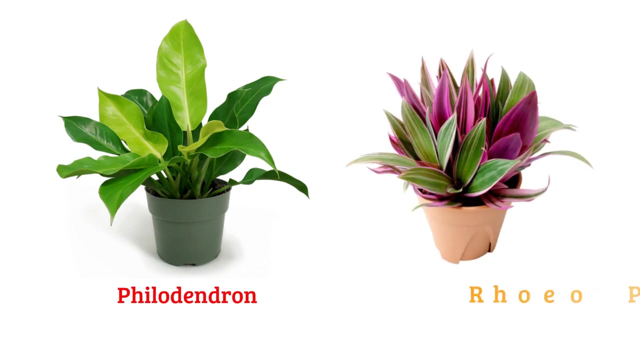 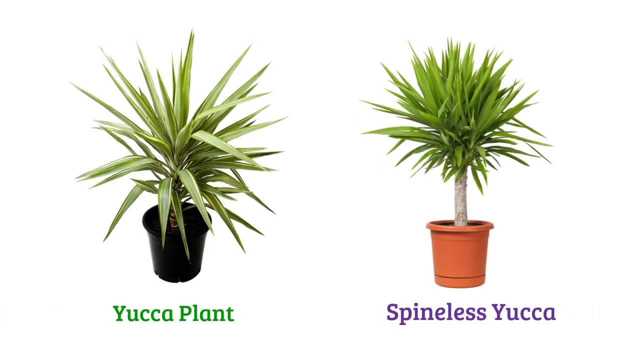 Holy Basil, Mother-in-law's Tongue. Aluminium Plant. Aglaonema Plant. Aralia Plant- Syngonium Philodendron Rio Plant. Yaka Plant- Spineless Yaka Dam, Cane Radiator Plant. 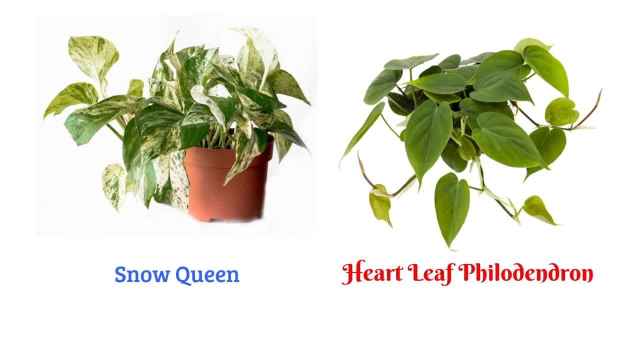 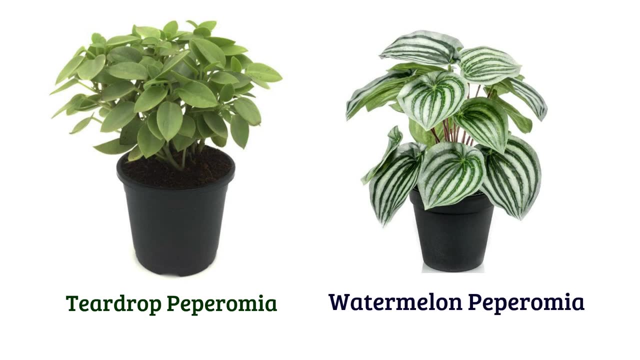 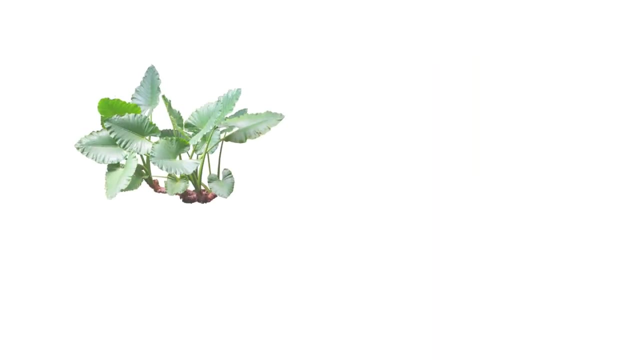 Snow Queen, Heartleaf, Philodendron, Teardrop, Peperomia, Watermelon, Peperomia Wandering Dew, Golden Pothos, Alocasia. O experiment on Breeze Cactus- Norking Garden. 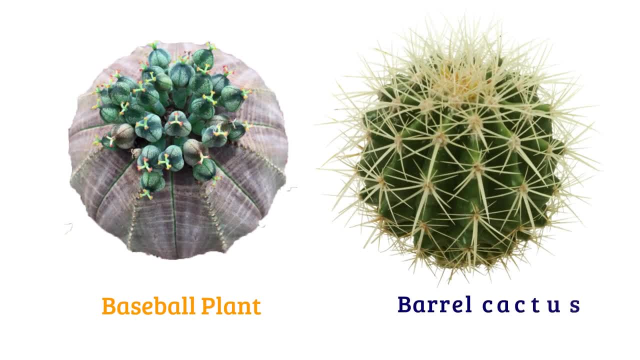 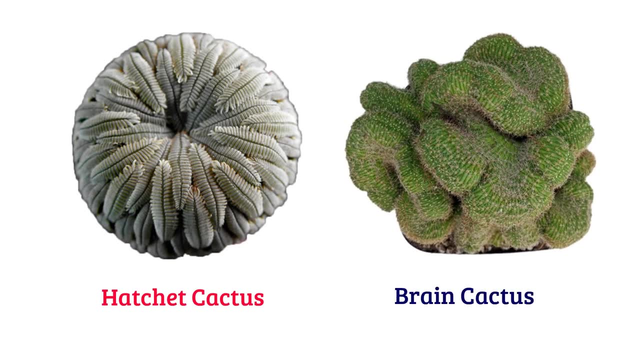 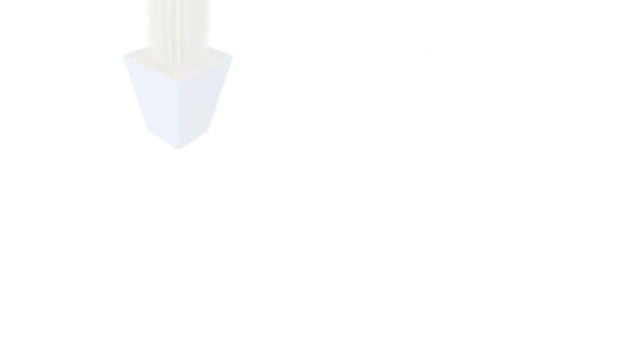 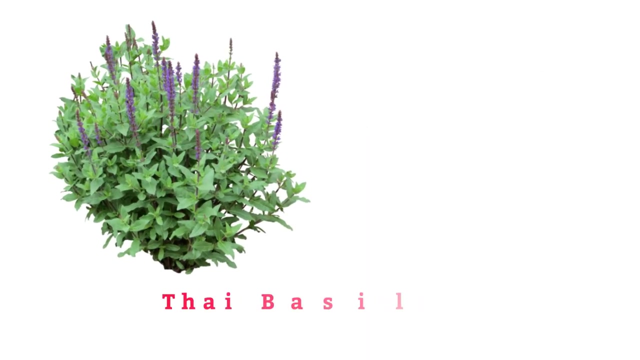 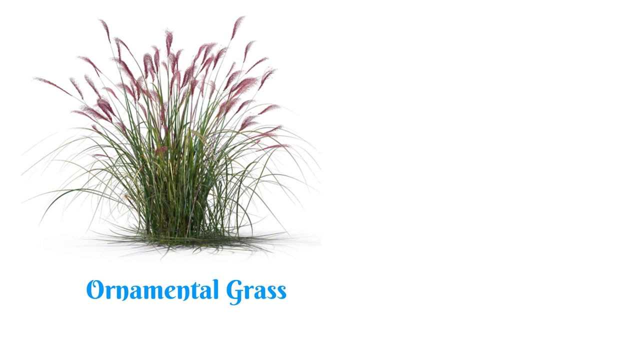 C помогids, disappointments, Aeternum position, reality, Serочка moment, the We have to Start 웠 Two englishоды. Plan Boo, covered plant. Criminal Completed Plant. Preis thousands, sundew plant. thai basil, livistona palm, ornamental grass, ruffled fan palm. 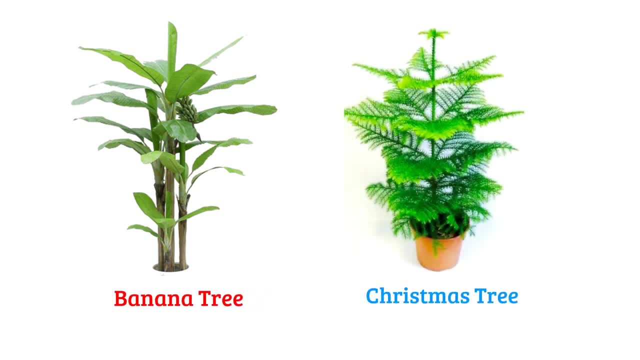 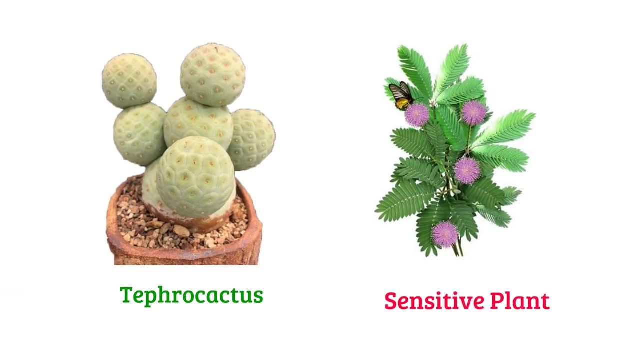 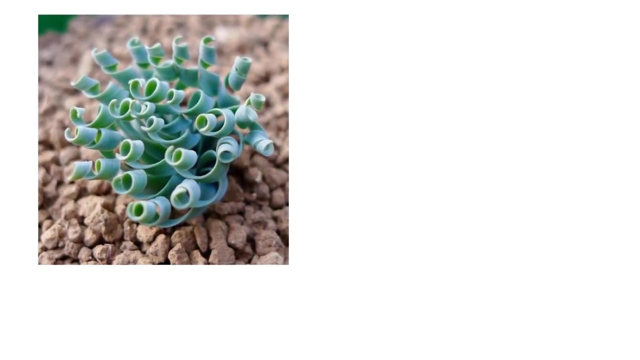 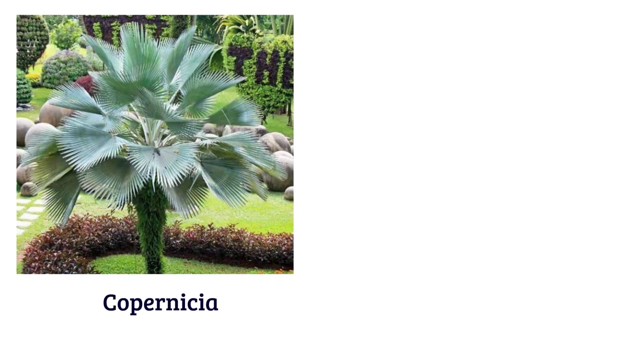 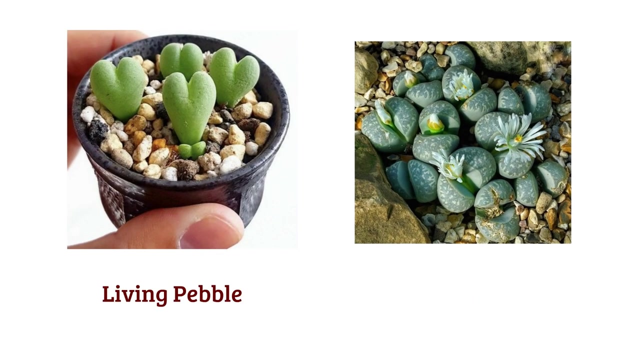 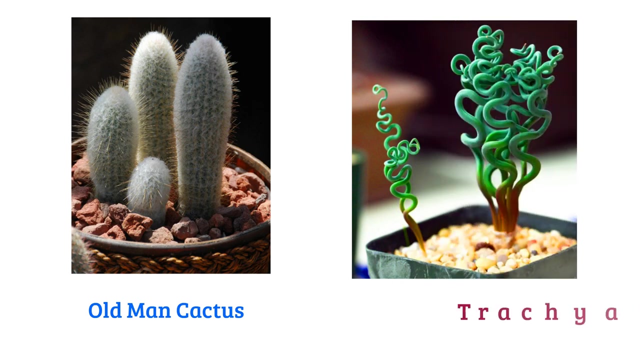 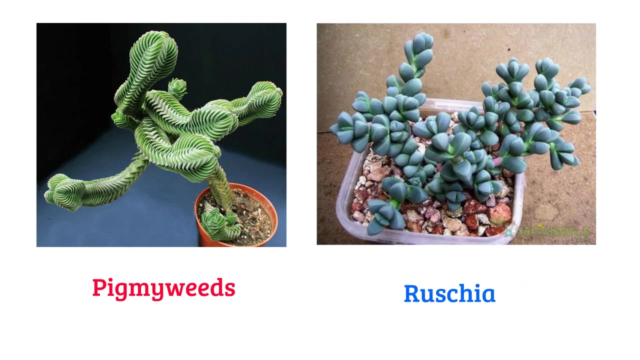 banana tree, Christmas tree, tephro cactus, sensitive plant, butterfly agave, bishop's cap, cactus albuca, carob, rose, copernica, blue agave, Living tree, Living tree, Living tree, Living pebble, living stone. old man cactus, trekkie, andra, pygmy, weed, ruskia thimble. 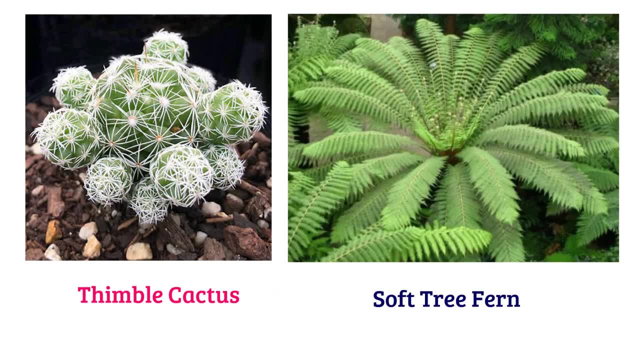